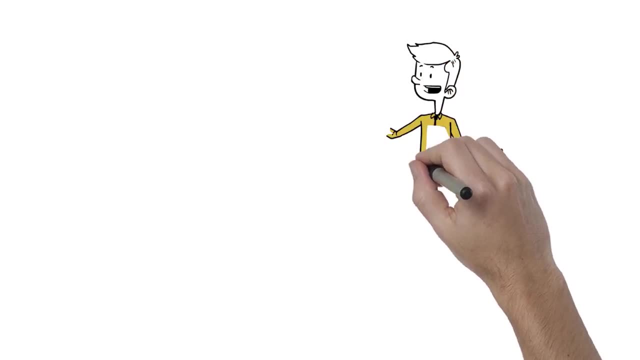 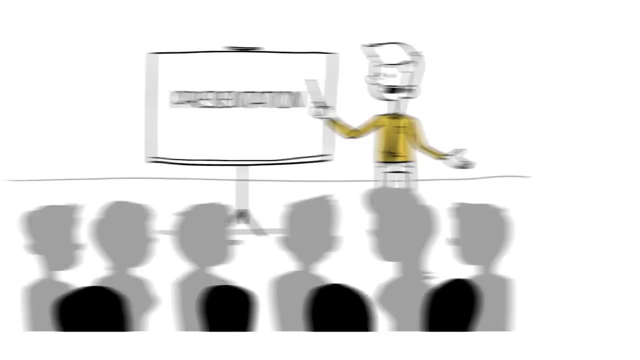 and design planning. A strategic meeting is then held, including the engineering team, AMP, quality and executive leadership, to finalize the project's scope and commit to bringing this product to market. And with a green light from our executive leadership, quality and AMP teams, our engineering 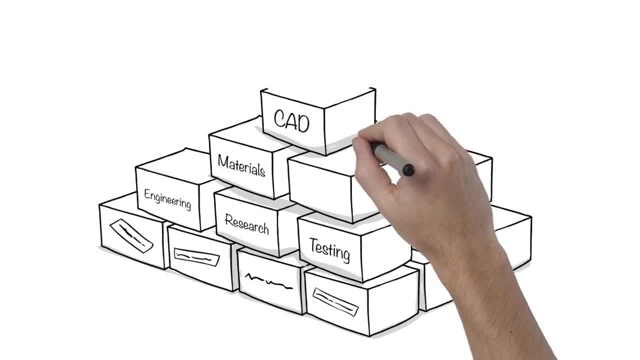 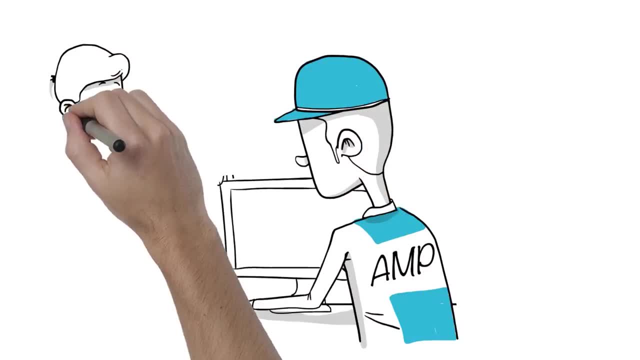 teams get to work constructing the building blocks that will become our new product, including final designs and test planning from the research team. Thank you, With the building blocks of the project in place, our engineering teams begin creating the first product with the finalized design, creating one or several working prototypes. 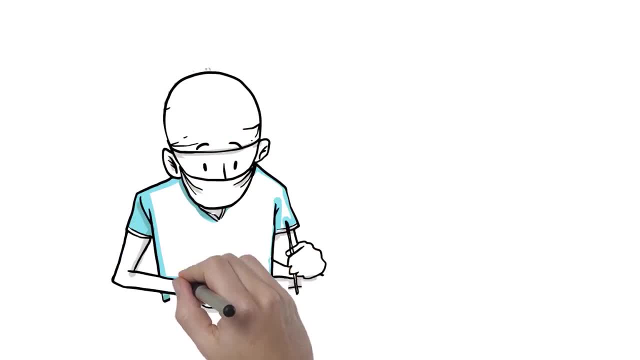 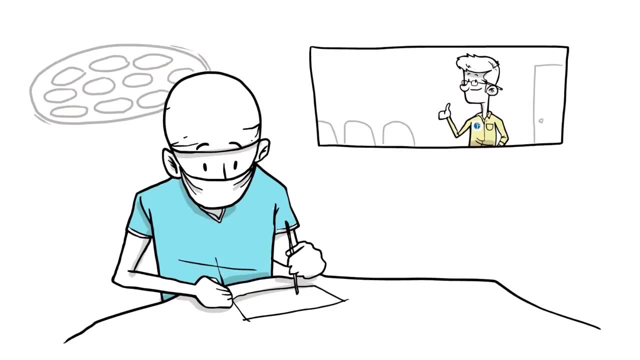 With these working prototypes in hand, our surgeon advisors, including CEO Dr Ching, can test the product during our clinical review process, testing the product's performance and effectiveness in a true-to-life scenario. With a thumbs-up from our surgeon advisors, our supply chain team can then source and. 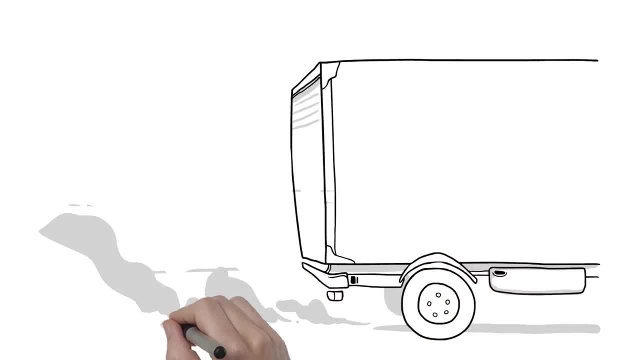 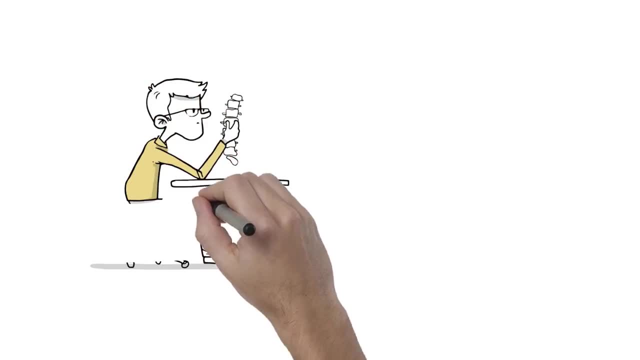 order our first batch of the new surgical system, bringing the design from concept to finished product. And if we're done yet, Once our manufacturing order arrives, our research and testing team puts the products through extensive tests and trials, conducting research to ensure the safety and efficacy. 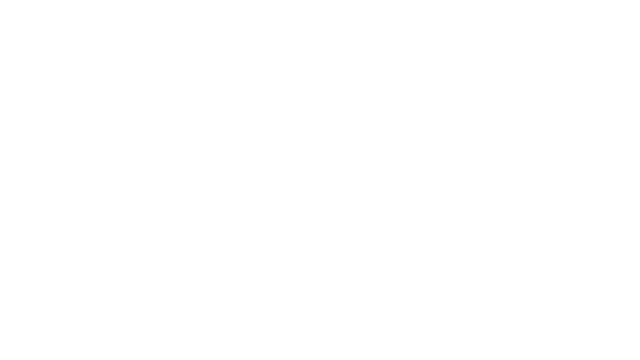 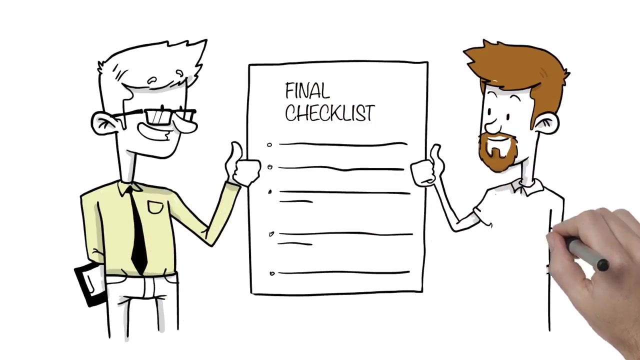 of each mechanism, part and instrument. With research and testing completed, our quality and engineering teams enter the final design review phase, ensuring every T is crossed and every I is dotted. This readies us for the most exciting stage in the process: delivering the final product. 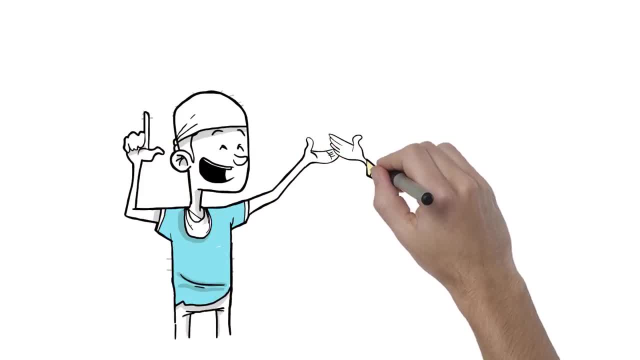 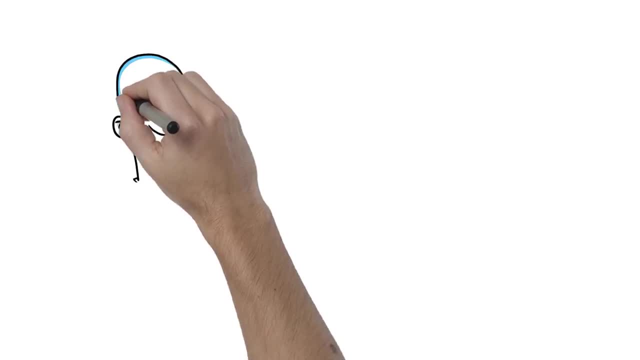 to our surgeon users- Yeah, We've received this idea at the beginning of the process- can now hold the finalized system in hand and use it to transform patients' lives for the better. But what if a surgeon has a custom request? As we know, each surgeon is different and each need is unique. 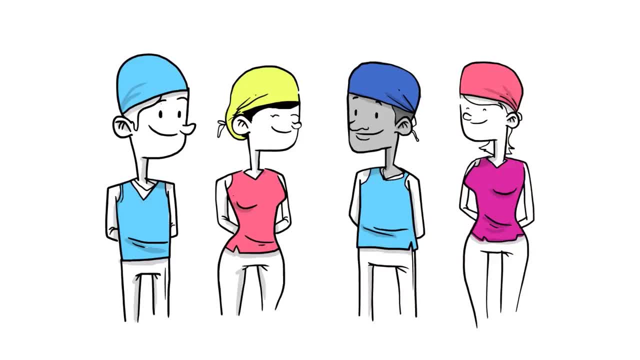 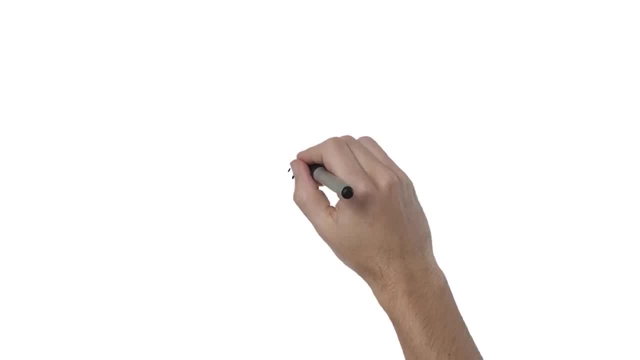 So, with this in mind, we've developed a process through which surgeons can submit individual requests for customized solutions. A surgeon simply submits their request to our product specialist engineering team, or PSET. Next, our strategic evaluation group comprised of executive leadership and sales management. 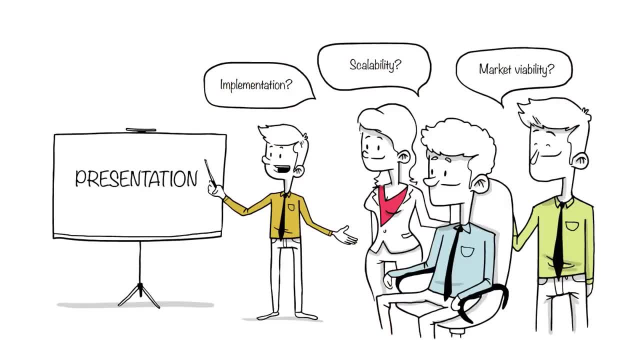 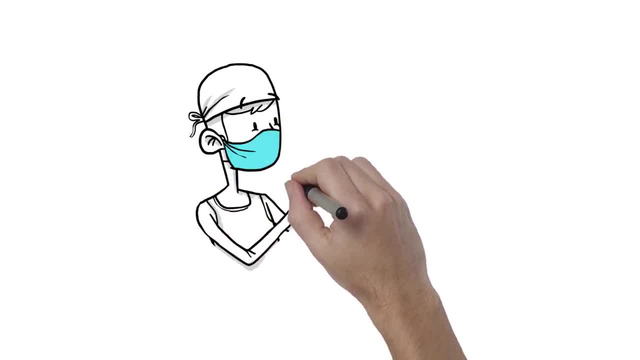 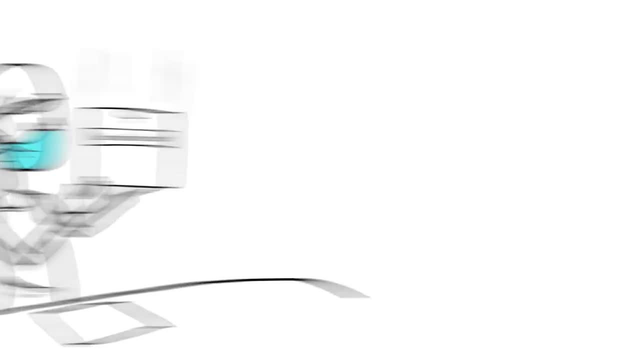 determine the implementation potential and the cost If this request remains an isolated project, our rapid customization engineering, or SPD, team facilitates the engineering process with speed and efficiency, getting the custom-tailored product back into the surgeon's hands as quickly as possible.